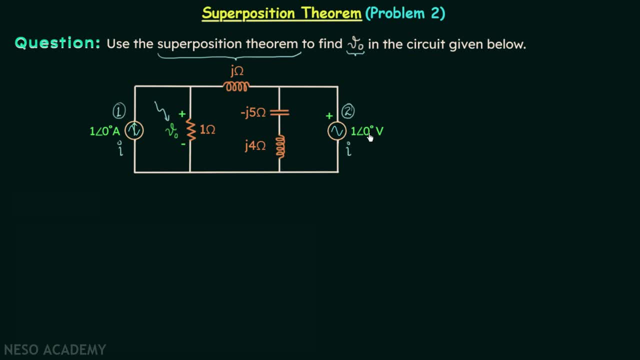 one ohm resistor because of this source, when this source is turned off, And then we will find out voltage across this resistor because of this source, when this source is turned off, And then, finally, we will add the two obtained voltages to have V0.. And apart from this, we are having one, two inductors and one. 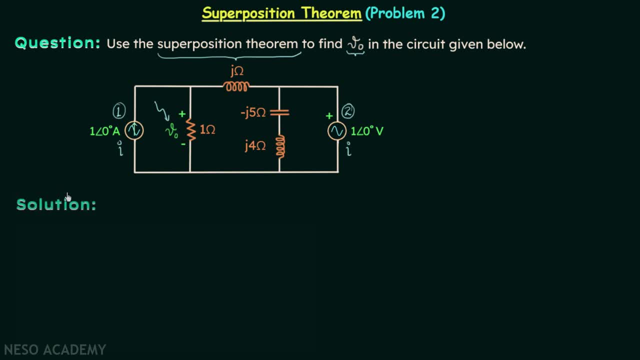 capacitor. Now we will move on to our solution And we will start with case number one, in which we will consider this source alone. we will consider one angle, zero degree ampere source. So let us start with this, Let's do the modifications to our network. The modification number one is we will replace the 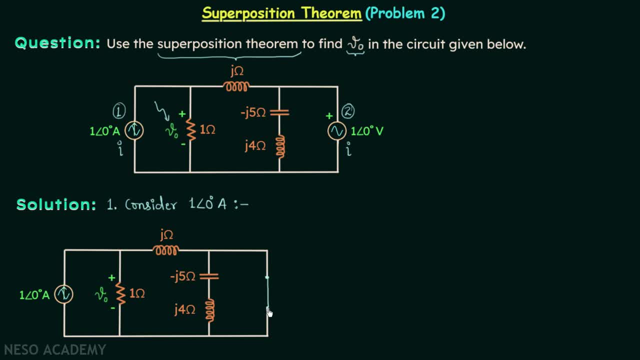 voltage source by the short circuit. And the modification number two is we will rename V0 to V0 prime And our aim in case number one is to find out V0 prime. And we can have V0 prime if we can have the current in this branch. Let's say the current is I1.. 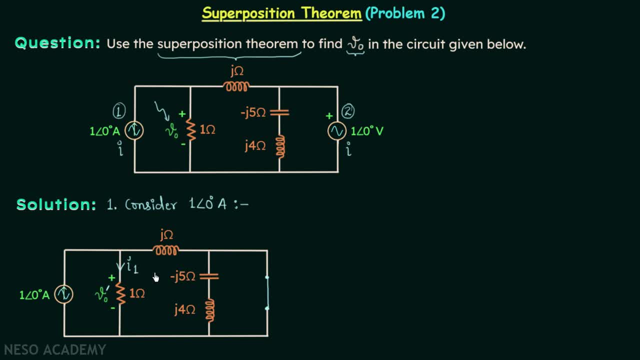 And to find out I1, we can use the fact that this resistor and this inductor are connected, in parallel connection, And the total current entering is equal to one angle, zero degree ampere. And why they are in parallel? because this branch, this branch is short circuited. This node and this 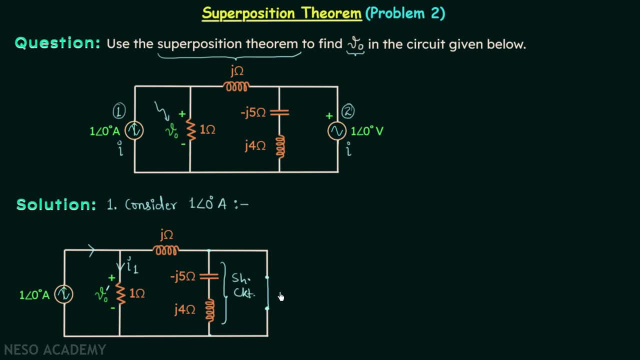 node are connected by the zero resistance wire and therefore, when current reaches this node, it will go entirely through this wire and not through this branch, because this wire is offering the resistance equal to zero ohm and the current will choose the path with least resistance and hence no current will flow in this branch, and it is short-circuited. now, moving on to 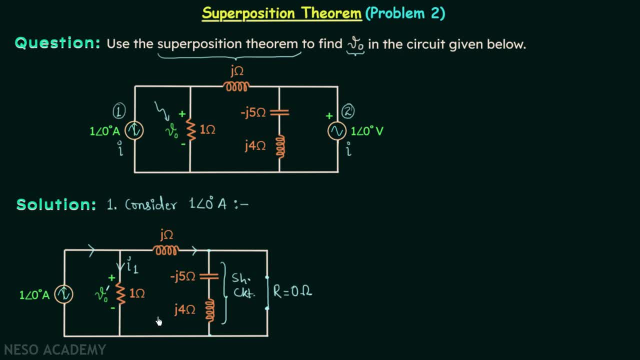 our parallel connection. we know in parallel connection current gets divided. so we can use the current divider rule. we can use the current divider rule. we know how to apply the current divider rule when there is a parallel combination. the current in this branch, which is I1, will be equal to the total current entering, which is one angle zero degree multiplied to the. 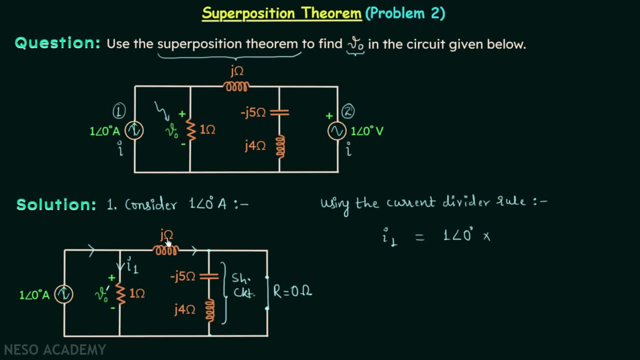 opposition offered by the other branch, which is J ohm, divided by the sum of opposition offered by this branch and the other branch, so we have 1 plus J, 1 plus J. now when you convert one angle, zero degree, in rectangular form, you will have 1. so I1 is equal to 1 multiplied to J over 1 plus J. so we can say that current I1. 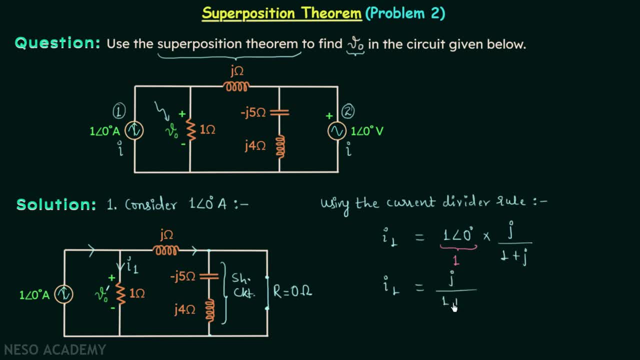 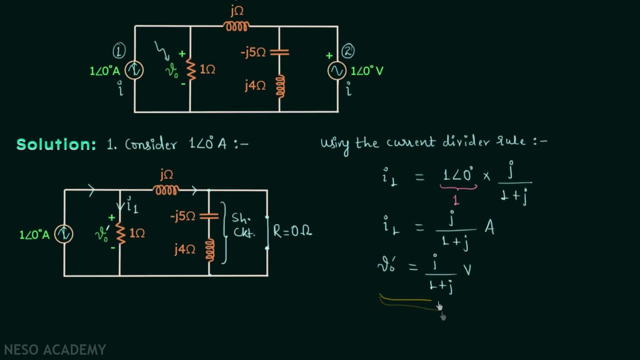 is equal to J over 1 plus J ampere and voltage, V naught prime is equal to I1 multiplied to 1 ohm. so we will have V naught prime equal to J over 1 plus J volt. so in this way we have obtained the voltage due to this source alone. now we will move on to our case. 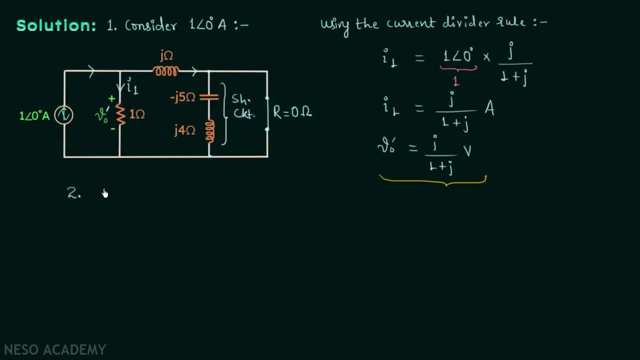 number 2, in which we will find out the voltage across 1 ohm resistor because of our source number 2. this means we will consider our source providing one angle, zero degree volt, and in this scenario, we will turn off our current source. so we will open our current source and we will turn off our current source, so we will open. 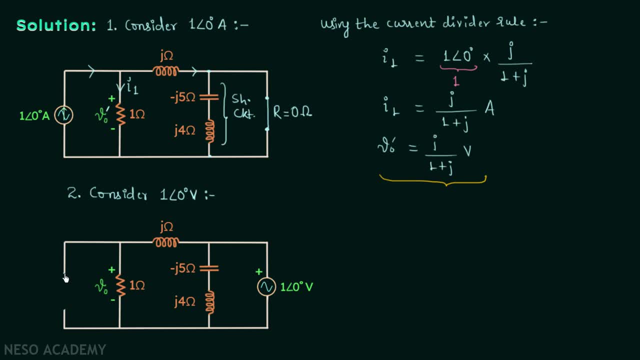 circuit the current source. this is our modification number one. the modification number two is we will rename V naught to V naught double prime. now let's see how we can calculate V naught double prime. and for this I will assume here the potential is zero volt. this means potential here will be one angle. 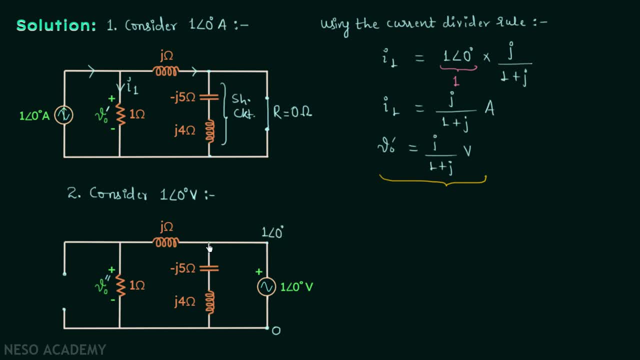 zero degree volt. potential here will become one angle. zero degree volt as well. potential here will be zero. potential here will be zero. this branch is open-circuited. this means if current I2 is flowing through this resistor, then the same current I2 will flow through this inductor. this means they are in. 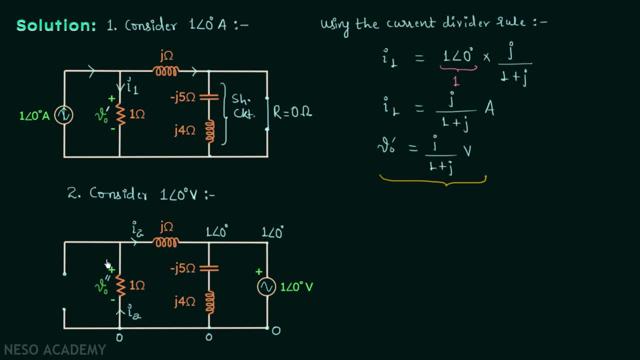 series combination and across this branch the voltage is one angle zero degree minus zero, that is one angle zero degree volt. so we have a series combination and we know the voltage across the entire branch so we can apply the voltage divider rule. so we will use the voltage divider rule to find out voltage V naught double prime, we know. 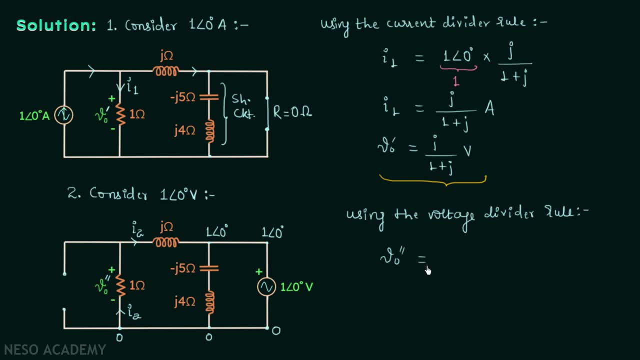 voltage V naught double prime will be equal to the net voltage across the branch, which is one angle zero degree, multiplied to the resistance offered by this branch, which is one divided by sum of these two, one plus zero plus J. in the rectangular form, one angle zero degree is equal to one, so V. 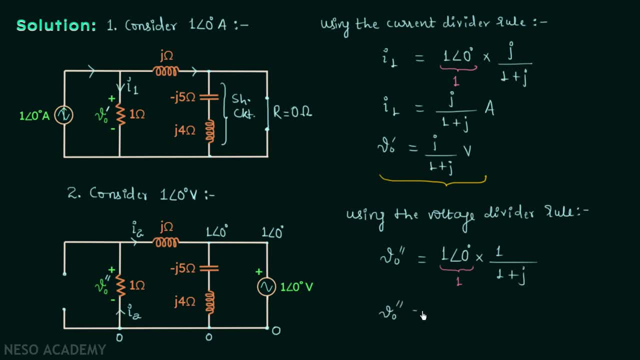 naught double prime. V naught double prime is equal to one over one plus J volt. so in this way we have obtained the voltage across one ohm resistor, because of our second source as well. now, by using the superposition theorem, V naught will be equal to negative zero. 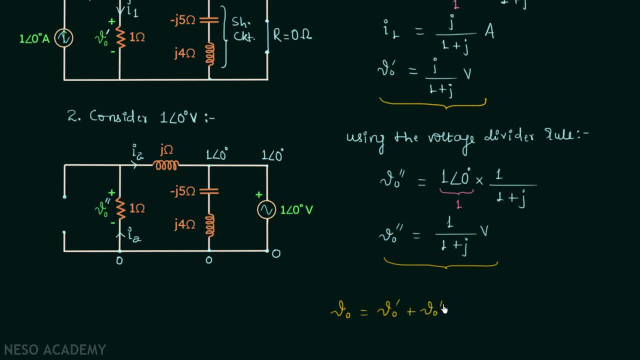 to v0 prime plus v0 double prime. This implies v0 is equal to j over 1 plus j, j over 1 plus j, plus v0 double prime, which is 1 over 1 plus j, 1 over 1 plus j. The denominator is same. 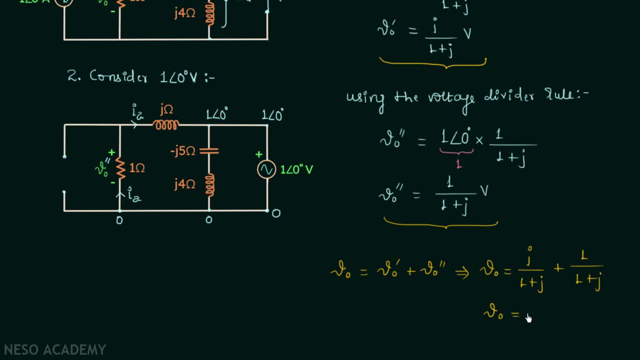 So we will have v0 equal to 1 plus j over 1 plus j, which is 1 volt. So this is the answer.